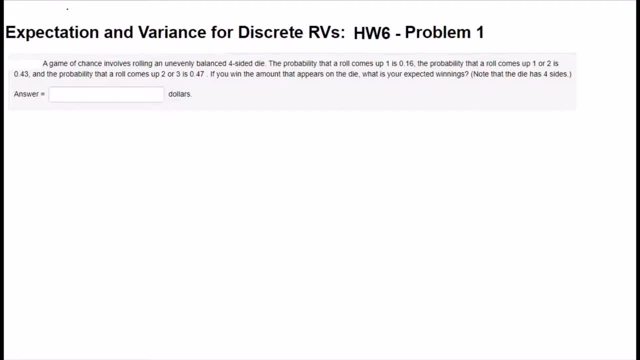 Hello everybody. In this video we are going to review expectation and variance of discrete random variables. This is problem number one. A game of chance involves rolling an unevenly balanced four-sided die. The probability that a roll comes up one is point sixteen. So let's write as we are reading. So 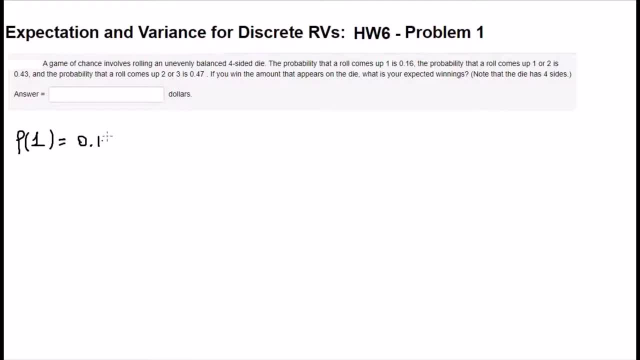 probability of getting one is point sixteen And we have four-sided unevenly balanced die. So we have numbers like one, two, three at the other side and number four in the bottom, like this, And the probability that a roll comes up one or two is point forty three. So the probability of one or two is point. 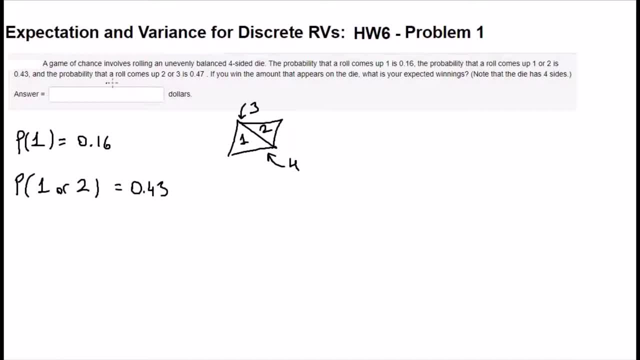 forty three, And the probability that roll comes up two or three is point forty seven. If you win the amount that appears on the die, what is your expectation winnings? So we're going to compute the expectation of this event. We know that each event is. 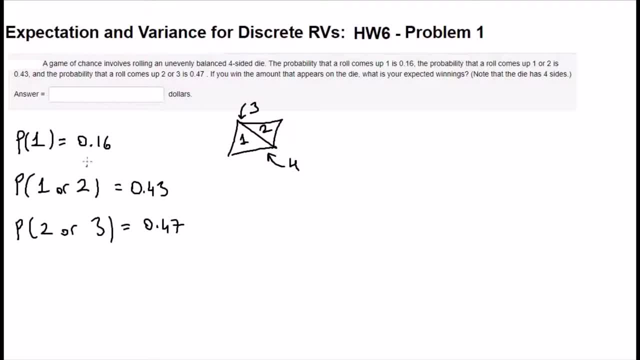 mutually exclusive, because two things here cannot have happened at the same time. Think like head or tails in a coin: It comes either head or tails. It doesn't come two of them at the same time, So this is mutually exclusive. So, knowing that this is mutually exclusive probability of two. 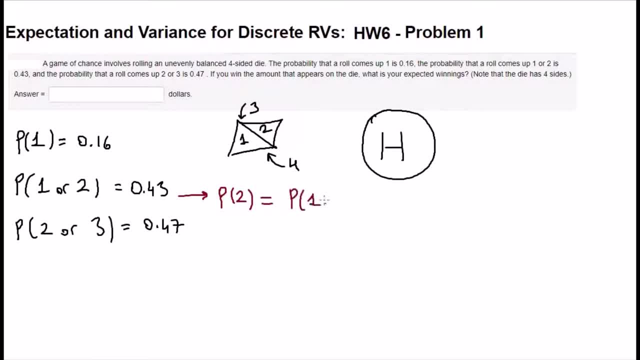 is equal to probability of one or two minus probability of one, And here, if we plug in numbers point forty, three minus point sixty and we'll give us point twenty seven. Similarly, probability of three is equal to probability of two or three minus probability of two, And if you plug in the numbers, point forty. 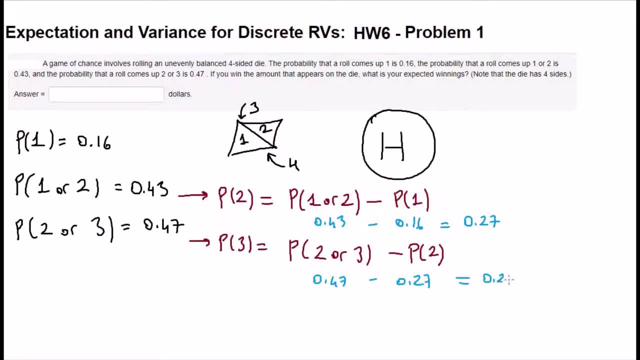 seven minus point twenty seven will give us point twenty. So how about probability of one of getting 4.. Probability of getting 4 is 1 minus everything, because total probability is equal to 1. So it will be 1 minus probability of 3 minus. 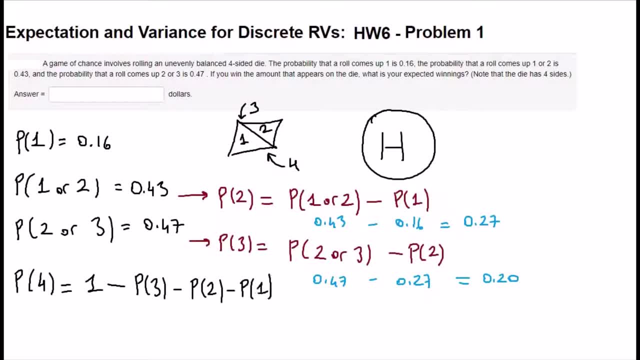 probability of 2 minus probability of 1.. And if you plug in the numbers, it's going to be 1 minus 0.20 minus 0.27, minus 0.16, 0.37.. Now we're going to compute. the expectation Expectation, by definition, is X times P the probability. 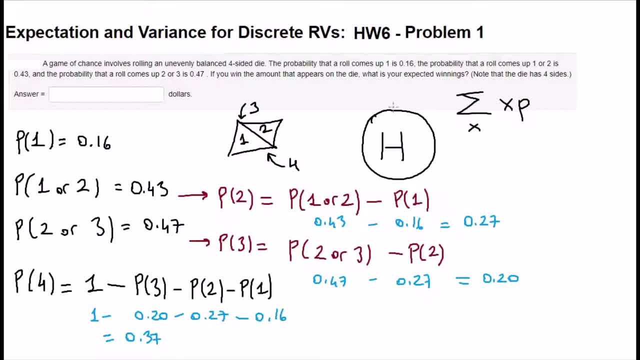 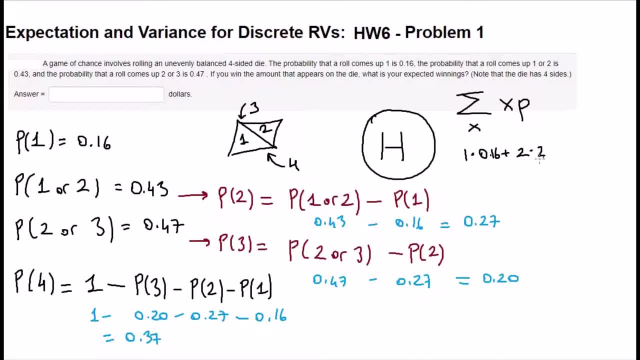 probability of 2 is 0.27 plus 3 times 0.20 plus 4 times 0.37.. So what we obtain is 2.78.. So the amount he makes is $2.78.. so the amount he makes is 2.78.. So the amount he makes is 2.78.. 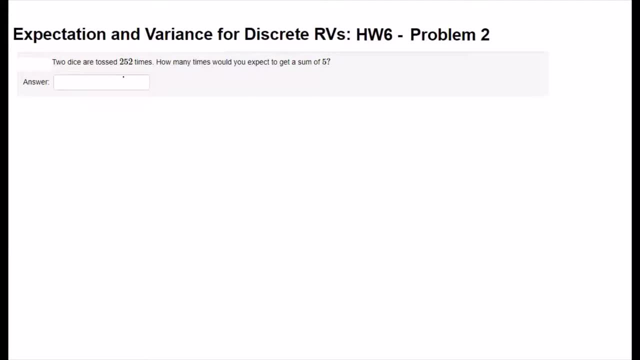 Problem numbers 2: to dice our toast. problem number 2.. Two dice are tossed 252 times. Problem number 2: to dice our toast 252 times. How many times would you expect to get a sum of five? Expectation is, by definition, Xi times Pi, which is the number of trial times. the 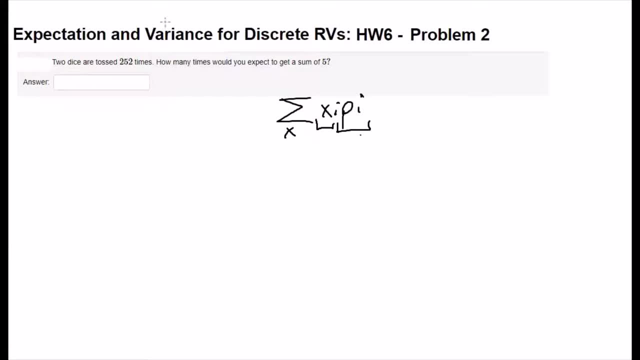 probability of that trial. We know that here our number of trial is 252 times. And we know that here our number of trial is 252 times. And we know that here our number of trial is 252 times. so now we're going to compute the probability of sum of five for single die. so probability. 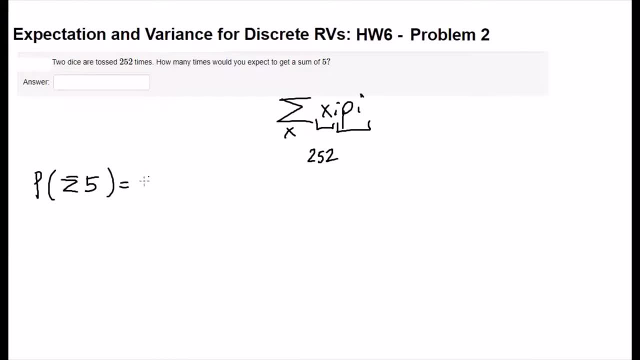 for sum of five is only given by. if we roll one and four and two and three and three and two and four, one, and if we combine these probabilities that's going to be the probability of getting sum of five. we know that probability of getting one is one. sixth probability. 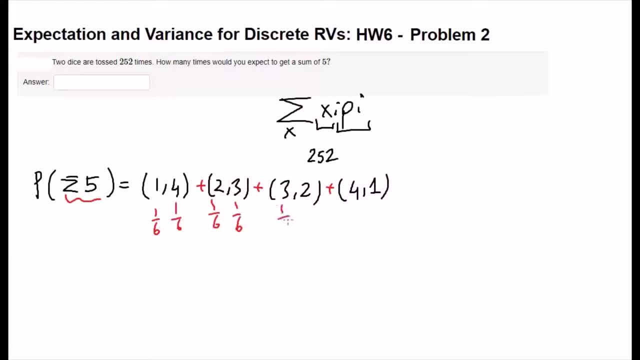 of getting each number is one sixth in a single die, and this probability will be one thirty six plus one thirty six plus 136 plus 136.. So that's going to be 4 out of 36, which is 1: 9th. So now we know that our p is 1: 9th, So the answer is 1, 9th times 252, which is x times p. 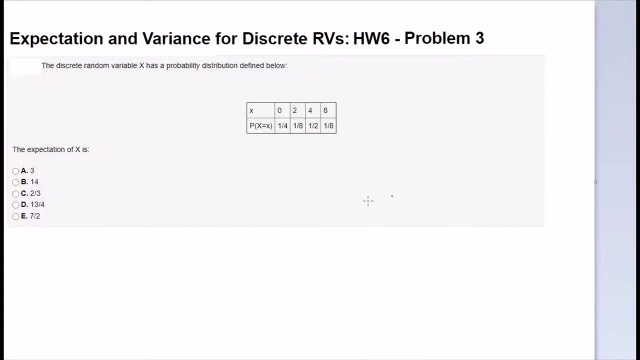 Okay, Problem number three: The discrete random variable x has a probability distribution defined below. So we're going to compute the expectation of this random variable x. Again: expectation, by definition, is the sum of x times the probability p, So it's going to be 0 times 1, 4th is 0, plus 2 times 1- 8th, which is 2, 8th. 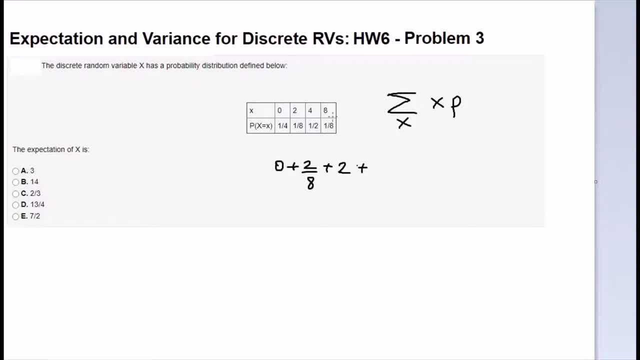 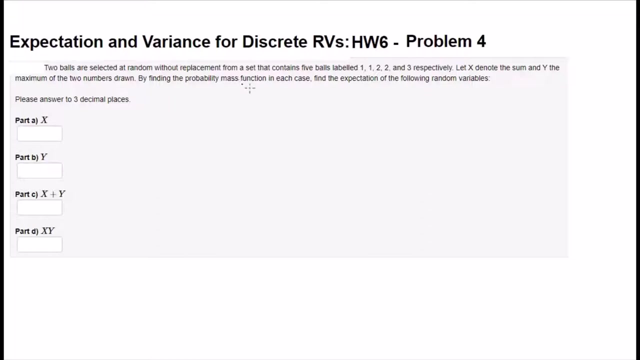 Plus 4 times 1 half, which is 2, plus 8 times 1 half, which is 1.. So if we add up all the probabilities, we obtain 13 over 4.. Problem number four: Two balls are selected at random without replacement from a set that contains five balls labeled 1, 1, 2, 2 and 3 respectively. 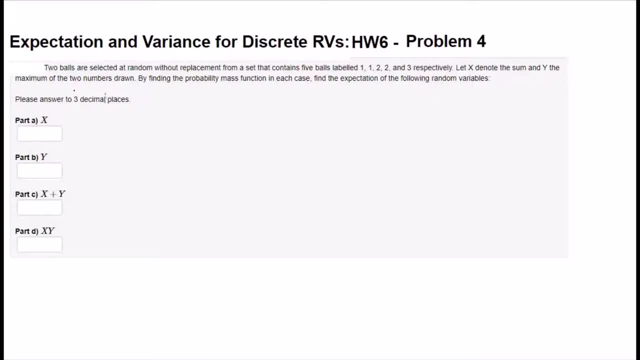 Okay, Let x denote the sum and y the maximum of two numbers drawn By finding the probability mass function. in each case, find the expectation of the following random variables: So here we're going to compute the expectation of x, y, x plus y and x times y. 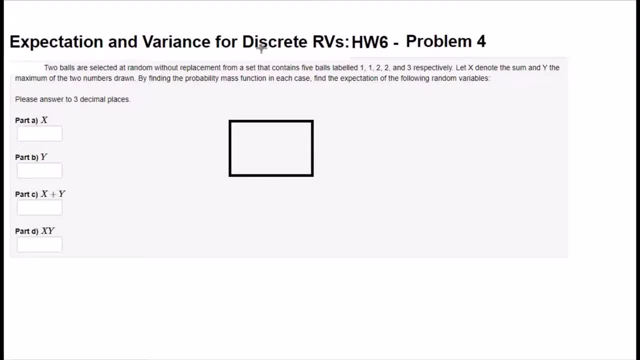 Let's illustrate the situation. We have a bag And in this bag we have the balls numbered 1, 1.. 2,, 2 and 3.. So we have five balls in the bag. So the probability of picking one is 2- 5th. 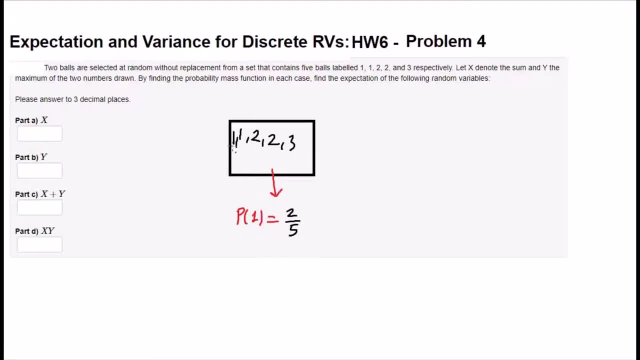 And probability of picking second one is: if we pick the second ball as one, it's going to be 1. 4th, because we do it without replacement. Probability of picking two Is again 2. 5th, because we have two, two balls out of five. 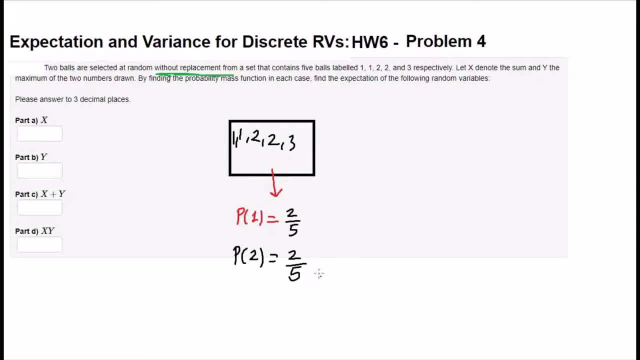 If we pick another ball two, it's going to be 1: 4th And probability of picking three is 1: 5th at the first coordinate. At the second coordinate, probability of picking three is zero because we have only one three. 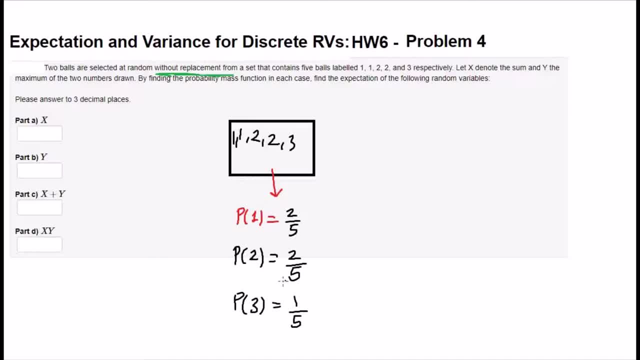 So we're going to use this information: X is denoting the sum Of two balls. We are picking two balls- And X is the sum of them, Coordinate one plus coordinate two. So the possible values of X is 2, 3, 4 and 5.. 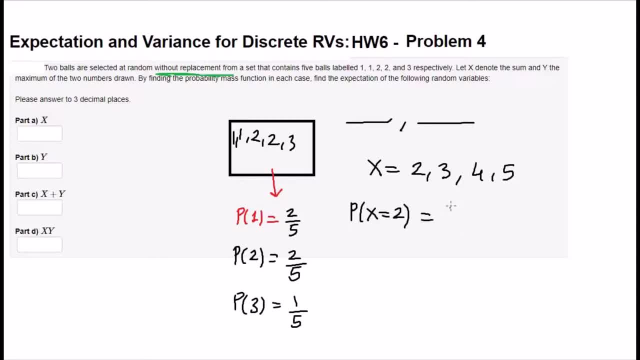 Probability that X is two is the only way that we pick one And then we pick again one. So 1 plus one gives us two. Probability that X is equal to 3.. Is two One, picking 1 first, then 2, or 2 first, then 1.. Probability that x is equal to 4: is we first? 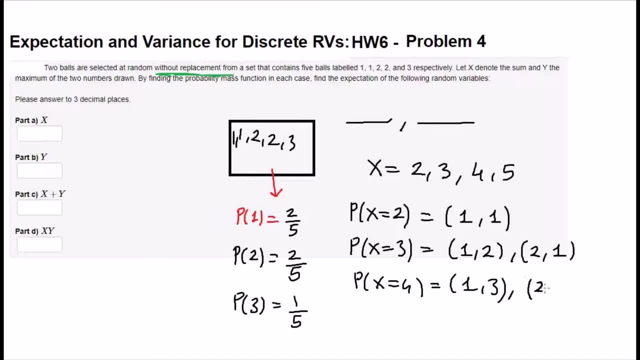 pick 1 and then 3, or we pick 2 and 2, or we pick 3 and 1.. And probability that x is equal to 5, that we first pick 2, then 3, or 3 and 2.. Now let's see the probabilities of each x here. 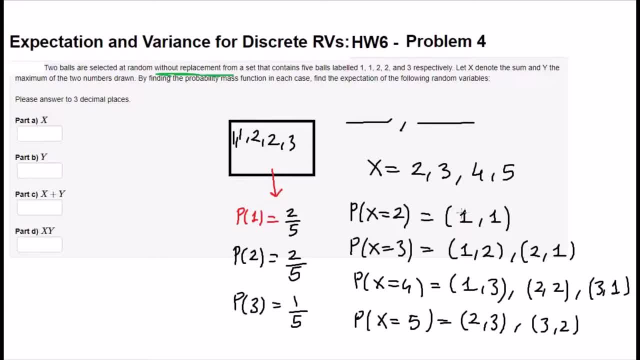 So probability that we pick 1 at the first coordinate is 2- fifth, And 1 again at the second coordinate is 1- fourth, without replacement, and we're left with 4 balls. Probability that we pick 1 and 2 is 1- fourth, And probability that we pick 2 and 3 is 2- fifth. 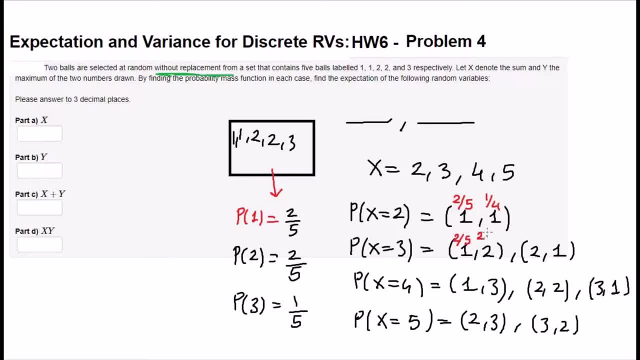 at the first coordinate is 2- 5th. this is 2- 4th and we're going to combine the probabilities here. picking 2 is 2- 5th and picking 1 is 2- 4th, 2 5th, 1 4th, 2 5th, 1 4th, 1 5th and 2- 4th. 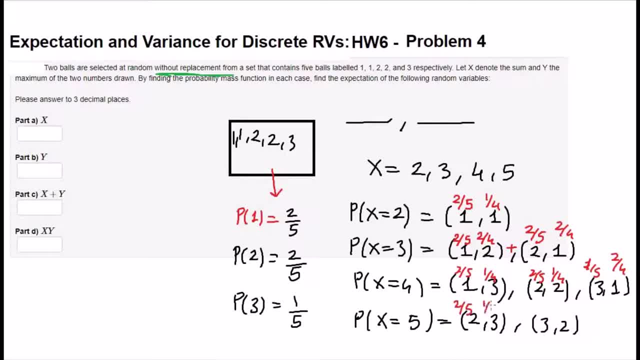 this is going to be 2- 5th, 1 4th and 1- 5th, 2, 4th, and we are combining the probabilities here. so the probability that x is equal to 2 is 2- 20th, and probability that x is equal to 3 is. 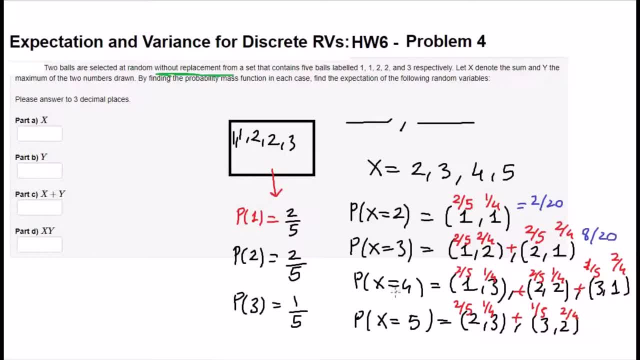 8- 20th. probability that x is equal to 4 is 2 plus 2 plus 2- 6- 20th. let's write it here: and probability that x is equal to 5 is 2 plus 2, which is 4- 20th. 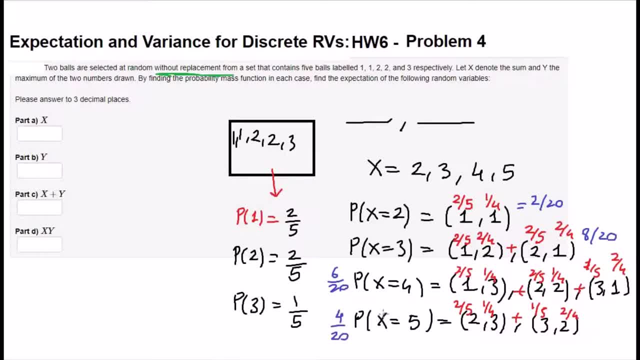 now, expectation, by definition is x times p- number of trial times, the probability that belongs to that x. so it's going to be 2 times 2- 20th. so it's going to be 2 times 2- 20th plus 3 times 8- 20th, plus 4 times 6- 20th and 5 times 4- 20th. so this is the answer. 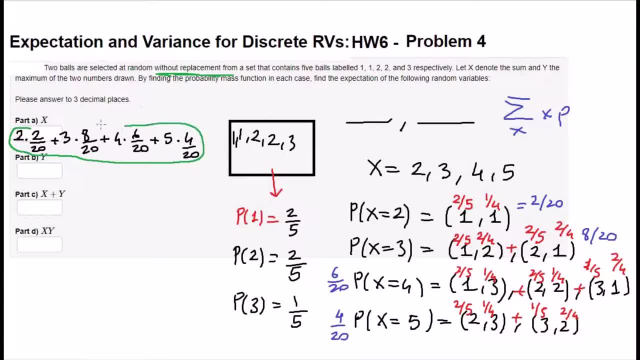 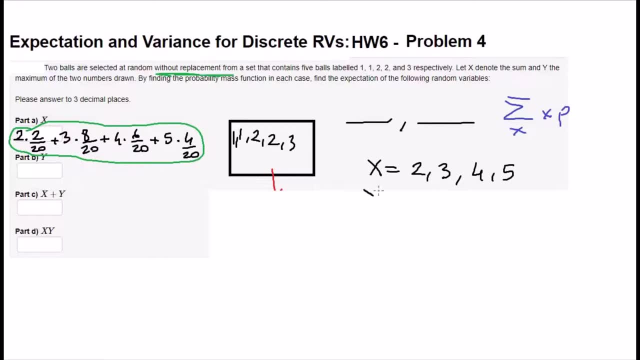 for: expectation of X. expectation of Y. let's clean up here. so this time we're going to write out the possible values that we can get for Y. Y is denoting the maximum numbers of two drawn, so we can minimum pick up one, two and three. those are the possible values for Y, probability that Y equals. 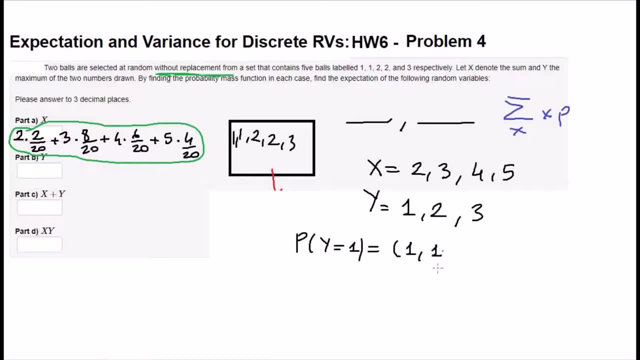 to Y is the only way we pick up one and one again. probability that Y equals to two is either we pick up 1 comma 2 or 2 comma 1 and the greater number is the value of X- I'm sorry- value of Y and probability that Y is equal to 3 is. 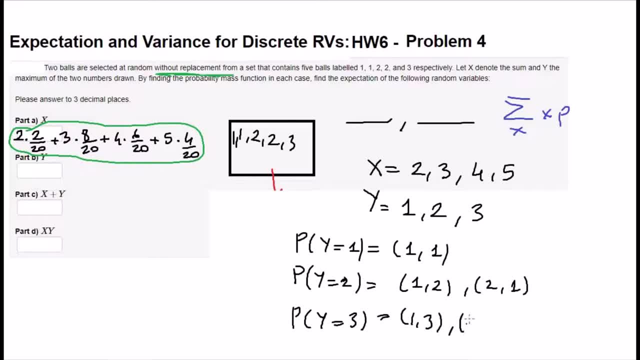 either we pick up 1 comma 3, 2 comma 3, 3 comma 1 or 3 comma 2. now let's see the probabilities of this and we're combining these probabilities. so picking one is 2, fifth, picking one is one, fourth, 2, fifth, 2, fourth, 2, fifth, 2, fourth, 2, fifth, 1, 4, 2, 5, 1, 4, 1, 5, 2, 4, 1, 5, 2. 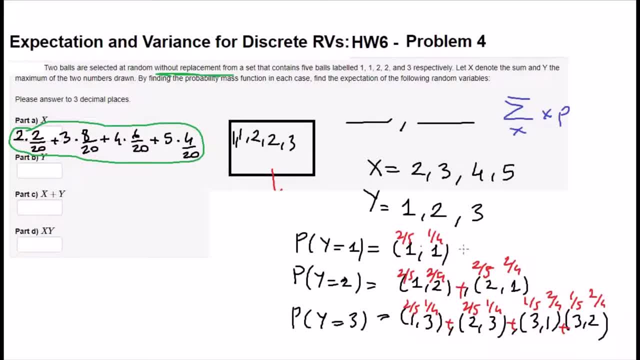 4th, and that y is equal to 1 is 2- 20th. this is going to be 2 times 2 is 4. 4 plus 4 is 8- 8- 20th. so this is going to be 2 plus 2 is 4 plus 2 is 6 plus 2 is 8- 8. 20th again, and expectation, by definition, is x. 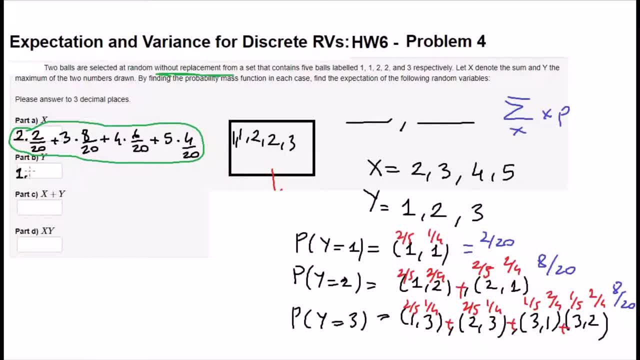 times p. so it's going to be 1 times 2- 20th, 1 times 2- 20th, plus 2 times 8- 20th plus 3 times 8- 20th. so this is the answer for expectation of y. 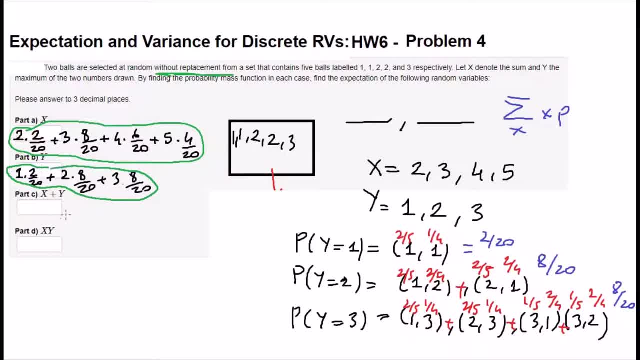 expectation of x plus y is the sum of these two expectations, because sum of expectations is equal to their addition. so so whatever value we obtain here, so expectation of x plus expectation of y, let's say we obtain here a and we obtain here b, so it's going to be a plus b, the values here. 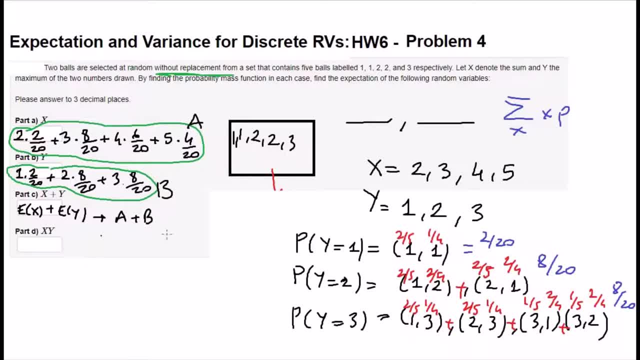 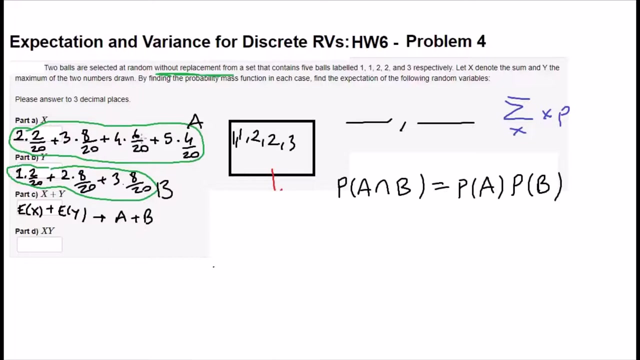 expectation of x, y will not be their multiplication, because those are not independent. how do we know that? because if we test for independency, let's do it here. simply, if two events are independent, their intersection is equal to their product. so let's test out one of them. 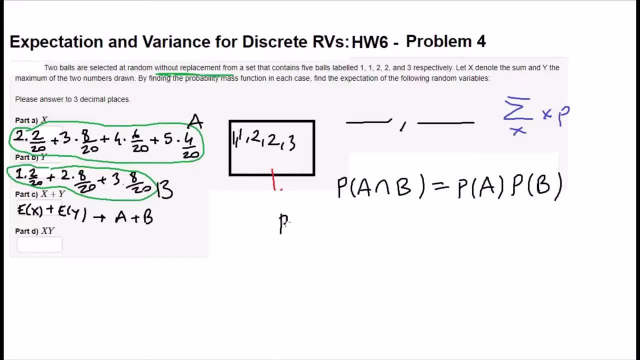 let's, for example, pick up that probability that X is equal to 3, probability that X is equal to 3 is 1 comma 2 and 2 comma 1 coordinates. and if probability of X is equal to 2, then probability of Y has to be 2 because the 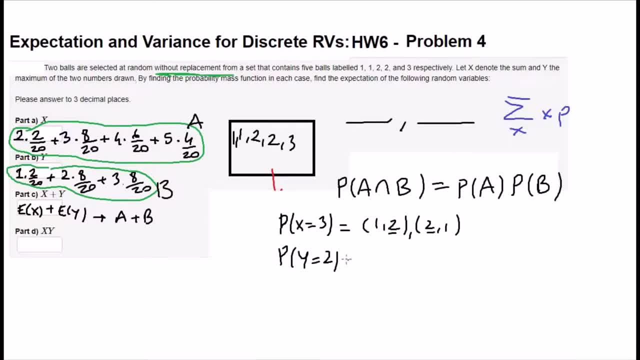 greater value is denoted by Y, and probability that Y is equal to 2 is 1 comma 2. probability that X is equal to 2 is 2 comma 1 and 2 comma 2, and probability that X intersect Y is, so only these are common, so it's 1 comma 2 and 2 comma 1. 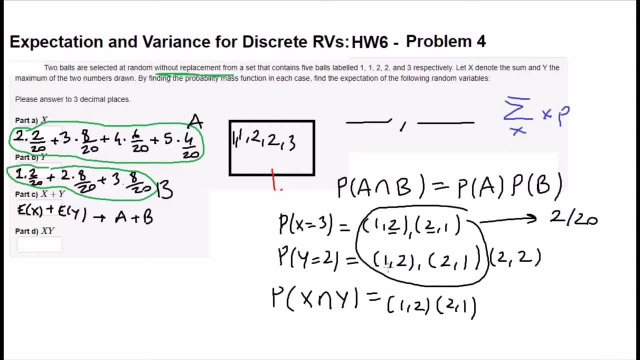 and probability that X is equal to 3 is: we've computed that it is 2- twentieth and we computed that it is 8- 20th, and this is 2- 20th and if we multiply 2 20th times 8, 20th. 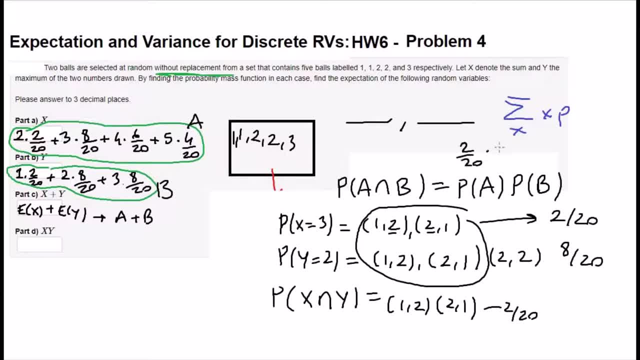 it is not equal to 2 20th. 2 20th times 8 20th is not equal to 2- 20th, so their product is not equal to their intersection. so we know that these two events are not independent. so now we are going. 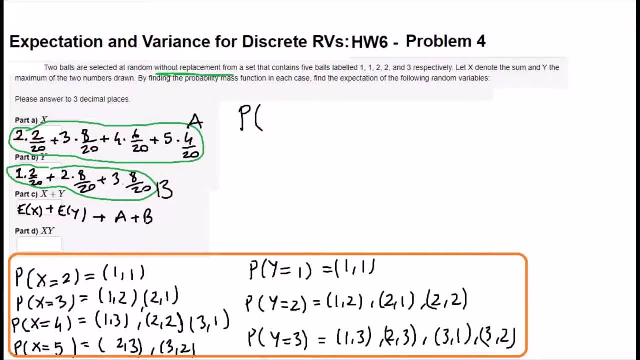 to treat this x times y differently. let's write out triple coordinates, so the first coordinate will be our x probability, the second coordinate will be y and the third coordinate will be x times y. so so probability that x is equal to 2 is only 1 and 1 in this case. the highest value here is 1, so y. 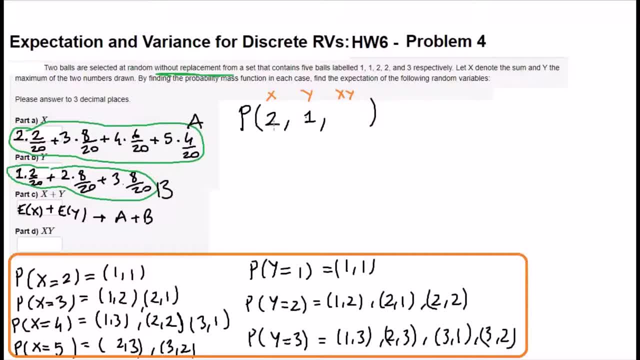 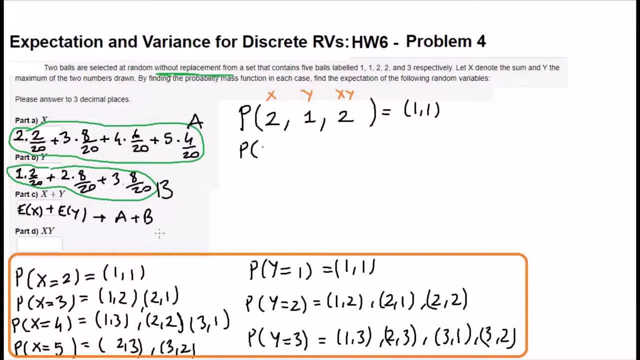 only 1 comma 1.. Probability that x is equal to 3 is only this: two coordinates, And in this case y will be 2, the highest value, And then x times y will be 6.. And that is only these two coordinates: 1 comma 2 and 2 comma 1.. Probability that x is equal to: 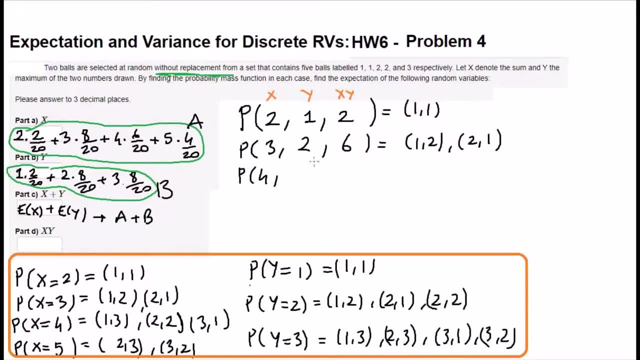 4 is only those three coordinates, And in this case the y value will be 3.. And x times y will be 12.. Here we need to separate this into two sections. We have y value 3, and we have y value 2 here. 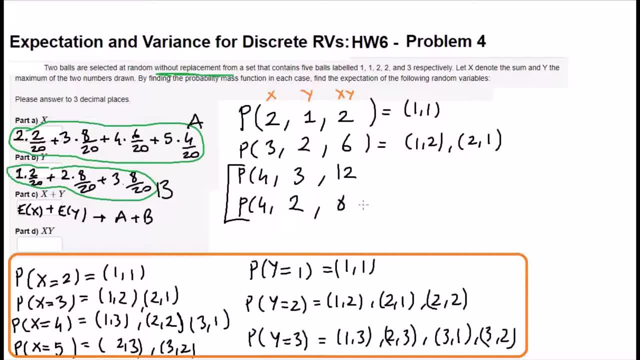 So in the coordinate 4 comma, 3 comma 12, our only coordinates are 1, 3 and 3, 1. And in this case our coordinates are 2 comma 2. And probability that x is equal to 5, then 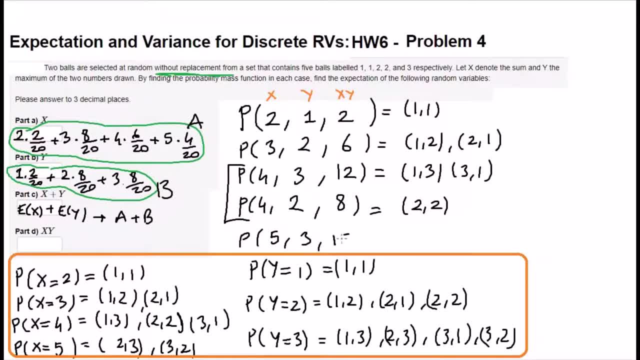 y value will be 3.. And x times y will be 15.. And only these two coordinates, only these two coordinates and only these two coordinates gives us this 5 comma, 3 comma, 15.. Now we can compute the probabilities here. So this is going to be 2 fifth times 1 fourth. 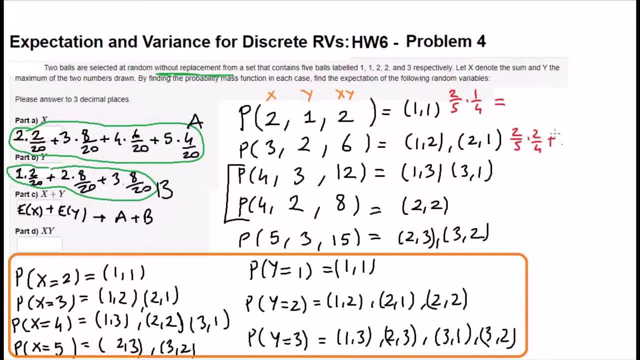 This is going to be 2 fifth times 2, fourth, So quarter times 1, quarter, Hopefully you fourth plus 2 fifth times 2. fourth. this is going to be 2 fifth times 1. fourth plus 1 fifth times 2 fourth. this is going to be 2 fifth times 1, fourth, and. 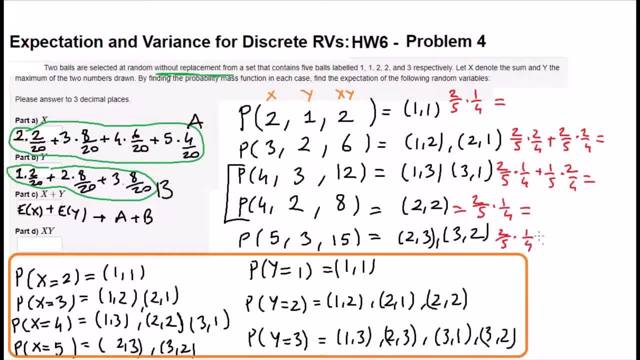 this is going to be 2- 5th times 1- 4th, plus 1- 5th times 2- 4th, and if we multiply, this is going to be 2- 20th. this is going to be 2 plus 3 is 4, 4- 20th. 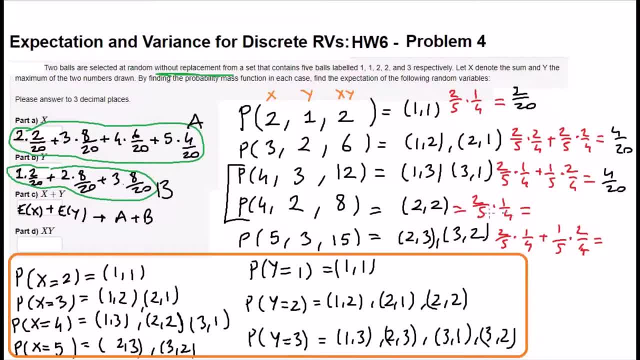 this is going to be again 4: 20th, this is going to be 2: 20th and this is going to be 4: 20th. now we can apply the definition of expectation so that by the definition of expectation we are going to multiply X times the probability P. so 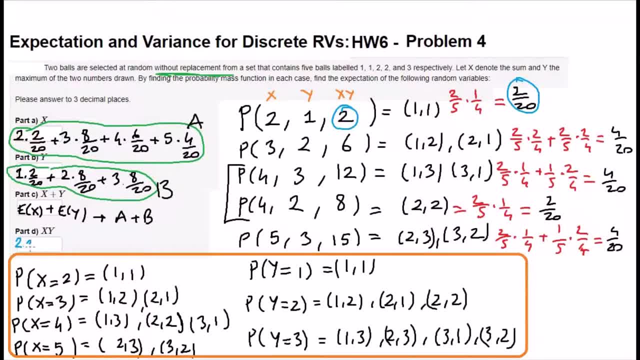 it's going to be 2 times 2- 20th, plus 6 times 4- 20th, plus 12 times 4- 20th, plus 8 times 2- 20th, plus 15 times 4- 20th, and this is the answer for expectation. 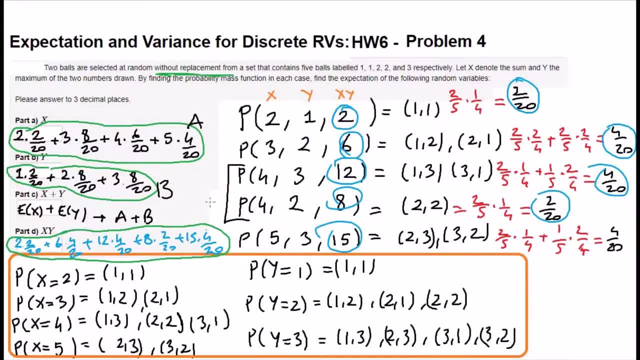 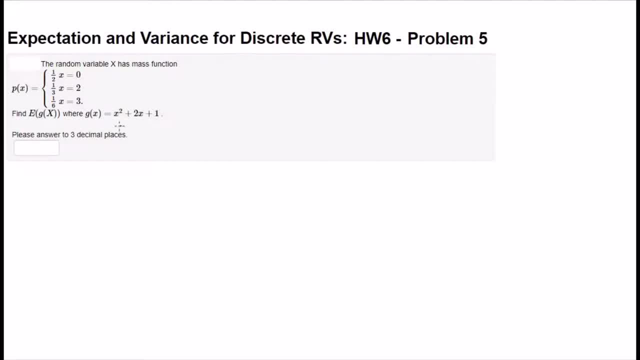 of X times Y, because these two events are not independent. problem number five: the random variable X has mass function given below. find E of G of X, where G of X is X squared plus 2, X plus 1. here we are going to compute the expectation. 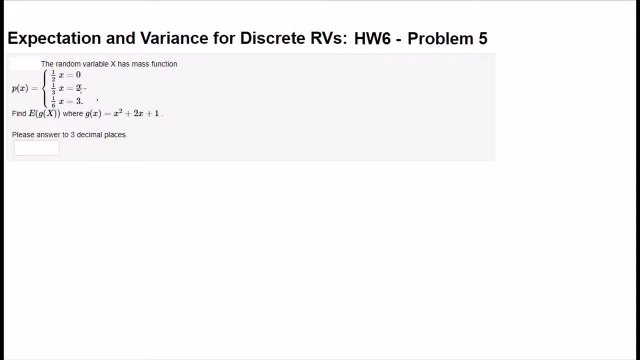 of a function. so we need to find the value of function at that given points. so we need to know what G of 0 is, G of 2 is and G of 3 is. G of 0 is, in this defined function, 0 squared plus 2 times 0 plus 1, which is 1. 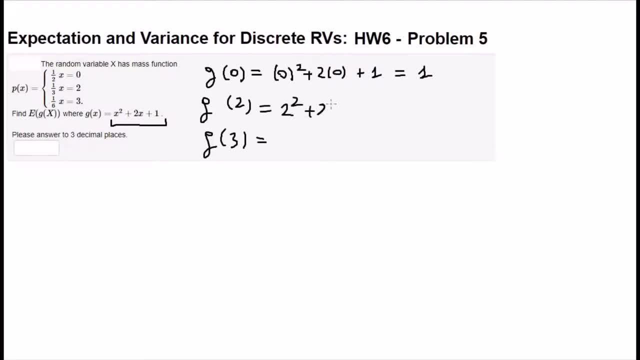 and G of 2 is 2 squared plus 2 times 2 plus 1, which is 9, and G of 3 is 3 squared plus 2 times 3 plus 1, which is 16, and we were given that 1 half X is. 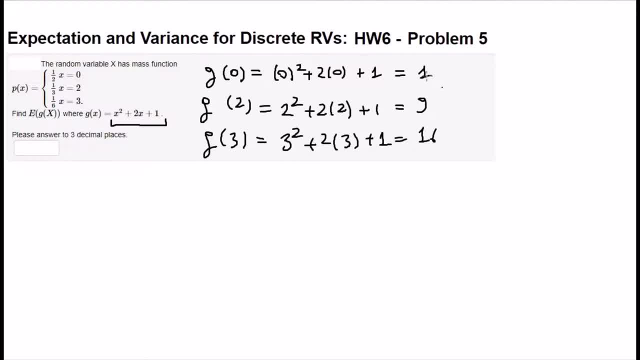 equal to 0 and G of 0 is equal to 1, so it's going to be 1 times 1, half, which is 1. half is equal to 2, and G of 2 is equal to 9. so 1 third times 9, which is 3, and for G, 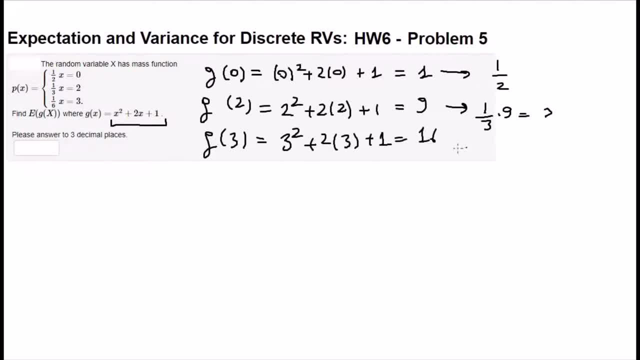 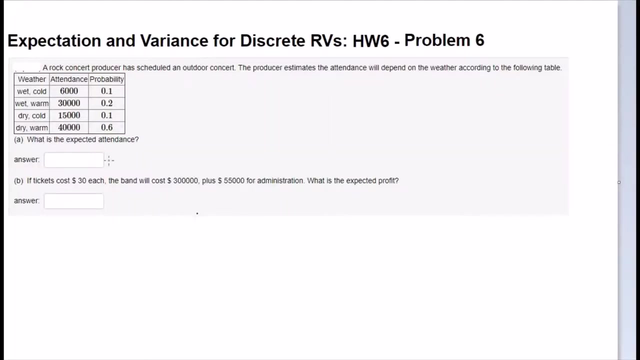 of 3, which is 16 times 1. sixth, which is 16 over 6, and if we combine these we obtain the expectation by definition. so one half plus 3 plus 16 over 6 is the answer. problem number 6: a rock concert producer has scheduled an outdoor. 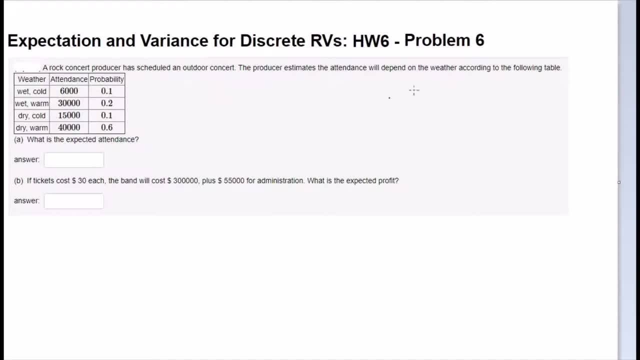 concert. the producer estimates the attendance will depend on the weather, according to following table. what is the expected attendance? again, by the definition expectation, it's going to be the sum of X times probability P, so it's going to be 6000 times 0.1 plus 30,000 times 0.2, plus 15,000 times 0.1 plus 40,000 times. 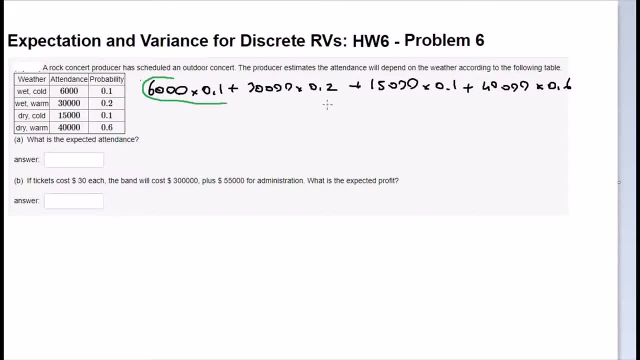 0.6 will be the mean or expectation. part B is asking: if tickets cost $30 each, the band will cost $30,000 plus $55,000 for administration. what is the expected profit? so for this, first we need to know what the mean is. so if we execute these numbers, it's going. 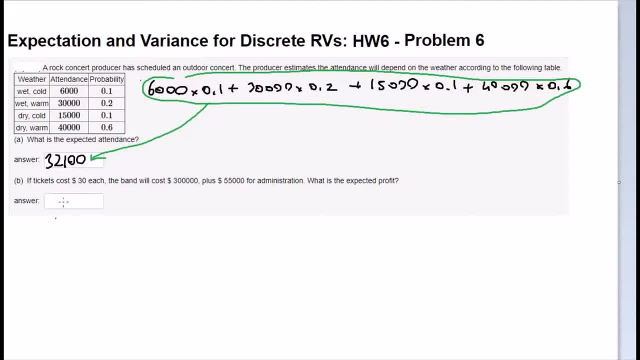 to be thirty two thousand one hundred and the total cost is $300,000 plus $55,000 and our total receipts will be the expectation or the mean number times the price of the ticket and expected profit, and will be this value, which is thirty two thousand one hundred times 30, minus the 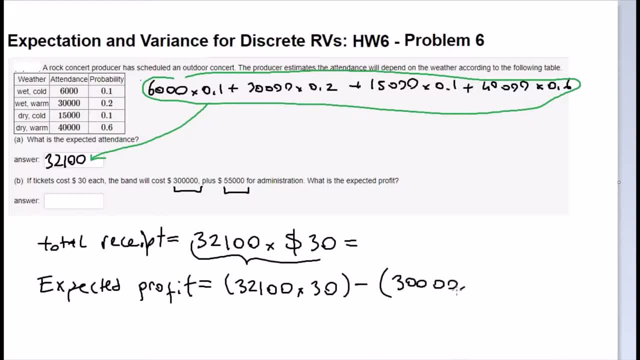 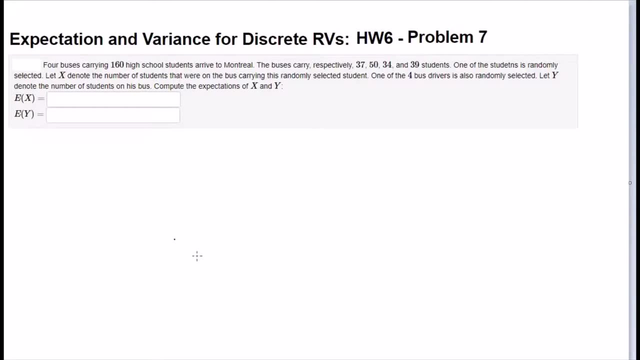 total cost. total cost is three hundred thousand plus fifty five thousand. so that's going to be the answer. problem number seven: four buses carrying 160 high school students arrived to Montreal. the buses carry respectively 37, 50, 34 and 39 students. one of the 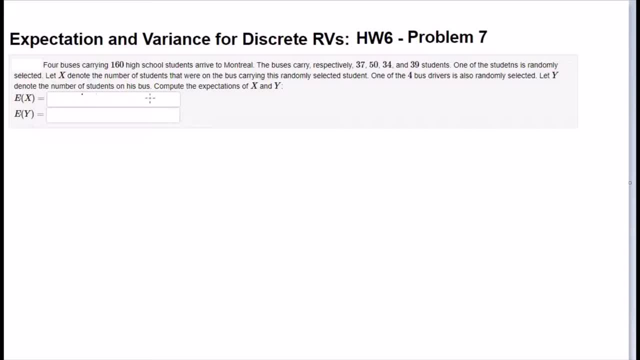 students is randomly selected. let X denote the number of students that were on the bus carrying this randomly selected student. one of the four bus drivers is also randomly selected. let Y denote the number of students on his bus. let Y denote the number of students on his bus. 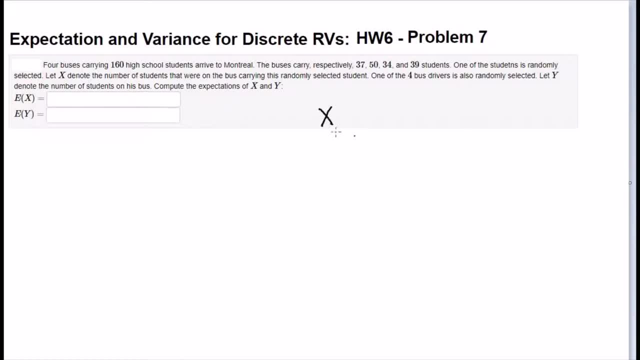 compute the expectations of X and Y, so we have 34ω, 37 am aye and 50 students are in each bus and the probability of this is 34 out of 160 and probability of death is 37 out of 160, similarly 39 out of 160 and 50 out. 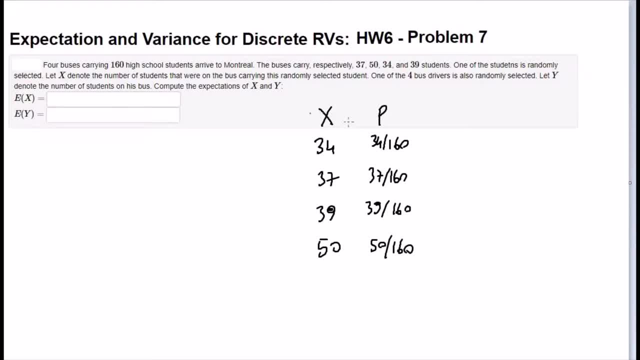 of 160 and, by the definition of expectation, X times P will give us the expectation. so the answer here will be 34 times 34 out of 160, plus 37 times 37 out of 160, plus 39 times 39 out of 160 and finally, 50 times 50 out of 160 will. 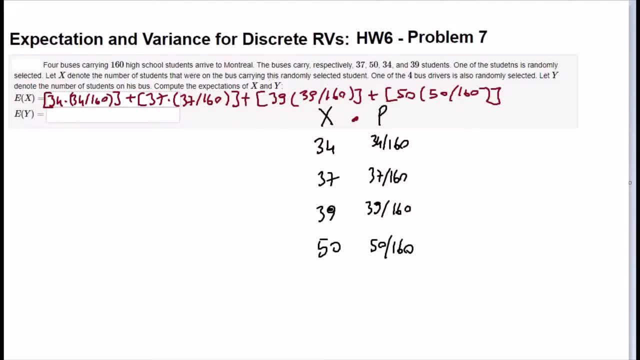 be the expectation for expectation of Y. again, we have same buses and same number of students, but this time probability of picking one of two the bus is one out of four, because we are picking the bus driver here and we have four buses and we are picking one of them, so it's 1, 4th and equally likely. 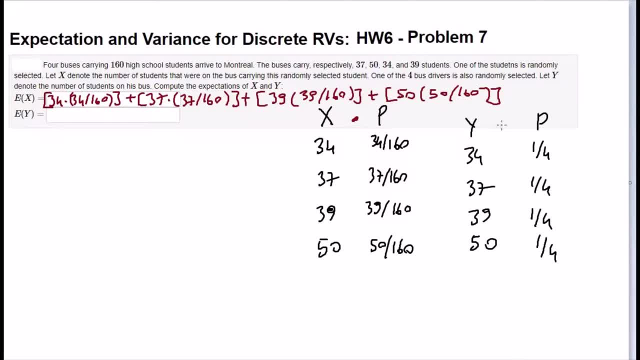 they are each 1 4th, and then expectation of Y, by definition, is going to be Y times P, which is 34 times 1 4th plus 37 times 1 4th, plus 39 times 1 4th, plus 50 times 1 4th, and if you would like to condense it, you can make it 1 4th. 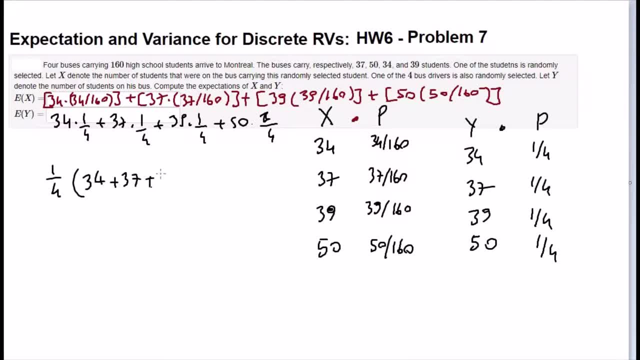 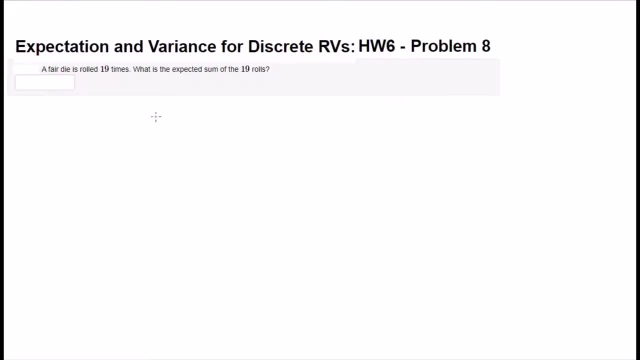 times 34 plus 37 plus 39 plus 50. problem number eight: a fair die is rolled 19 times. what is the expected sum of 19 rolls for a single die? our expectation it is a flat die roll. so the value of the die, that is, the expected value, is one. 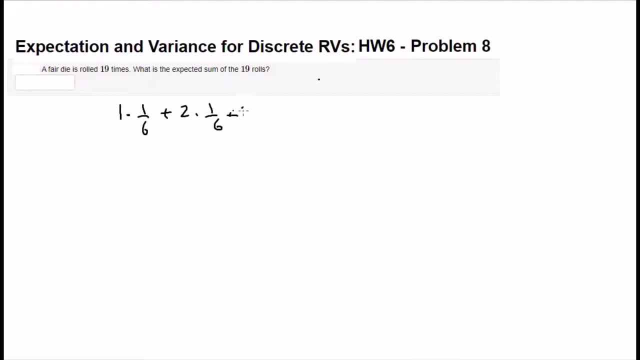 times 1, 6 plus 2 times 1, 6. that is the probability and the value of each number plus three times 1, 6th, 4 times 1, 6, 5 times 1, 6 and 6 times 1, 6, and we know. 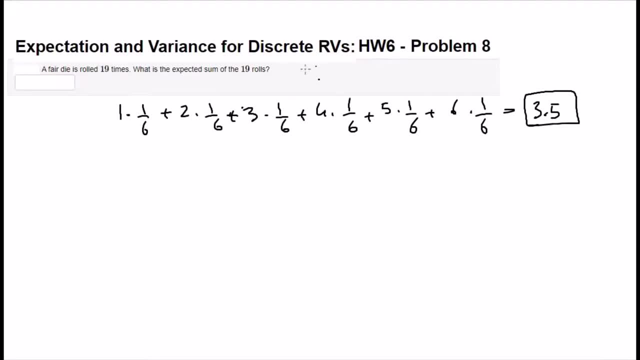 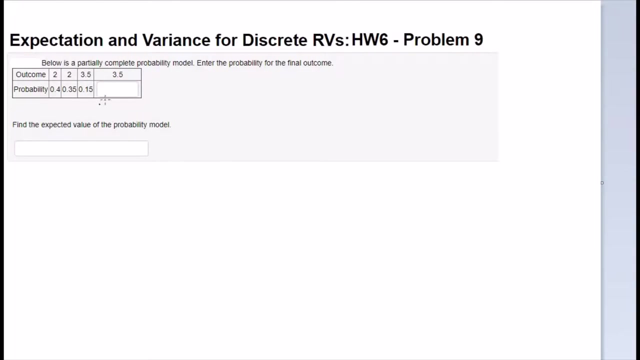 this by heart. it is 3.5 is the average expected value of a single die roll and times. so if we multiply 19 times the average value of single die, we obtain 65.5, which is the expectation of the sum of the 19 rolls. problem number 9 below is a partially complete probability. 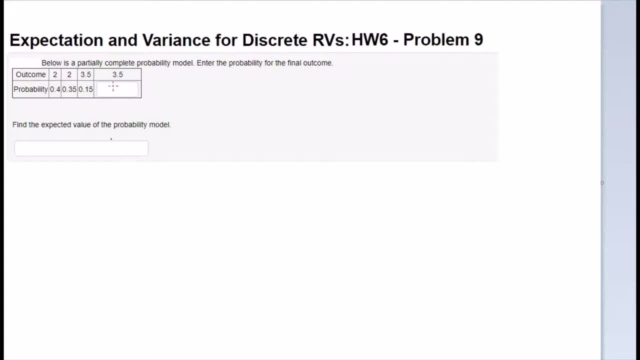 model enter the probability for the final outcome. so for this gap we know that the total probability is equal to one. so one minus everything, which is 75, 80, 90. so this is going to be 0.1, because that's the number that completes to one, and expected value by definition is x times p. outcome times. 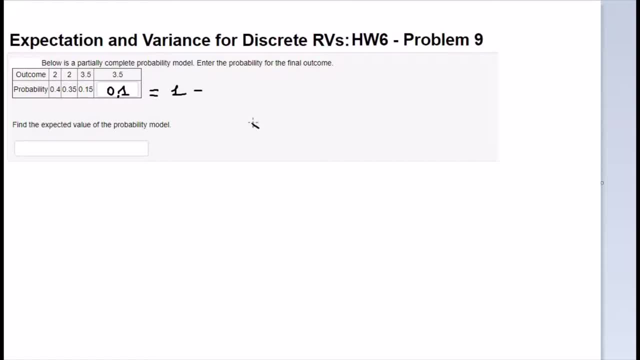 the probability. so 2 times 0.4, which is 0.8, 2 times 0.35, which is 0.7, plus 3.5 times 0.15, plus 3.5 times 0.1, and this is going to be answer. 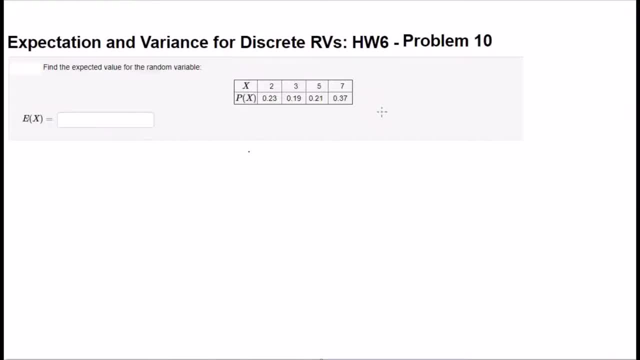 for the expected value. problem number 10: find the expected value for the random variable expectation. by definition is outcome x times the probability of that outcome. so here we were given explicitly in the table. so it's going to be 2 times 0.23 plus 3 times 0.19 plus 3 times plus 5 times 0.21 plus 7 times 0.37. 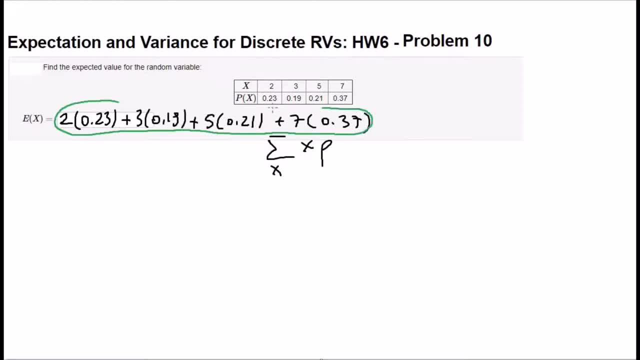 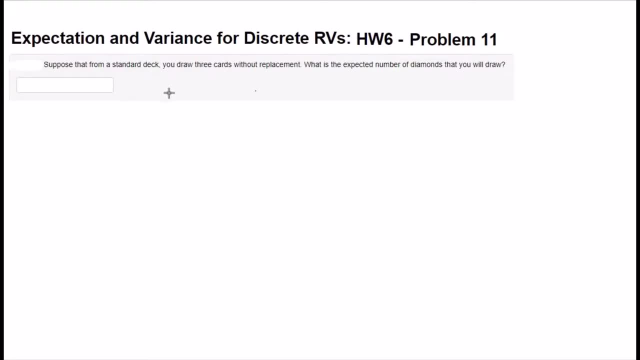 so this is the expected value for this random variable x problem, number 11. suppose that from a standard back you draw three cards without replacement. what is the expected number of diamonds you will draw in this problem? we need to know first the number of diamonds. so we have 52 cards in standard deck. 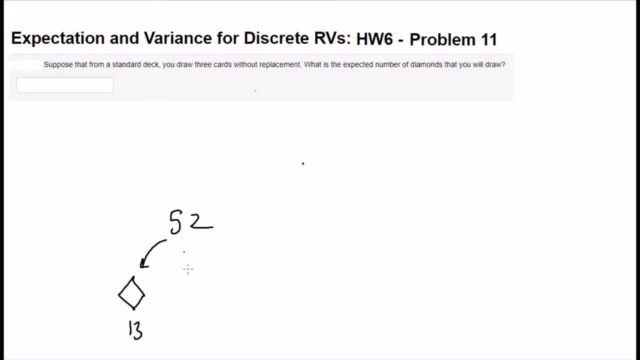 and 13 of them are diamonds and the rest three other suits are 39 cards, 13 plus 13 plus 13.. so for the first card we are picking is the probability is 13, choose one. and non-diamond cards are 39. choose the rest two, because we are picking totally three cards. 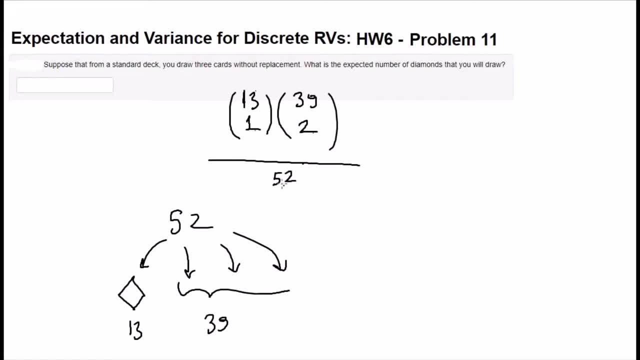 and our total number of combinations is 52: choose three. so we can formulate the random variable with a three card method. let's go with this method. so if we choose three of the flushed cards and we have the correct answer in the next three cards, we are gonna choose imperial, and then we have the three of the two in the next three cards, which is left as the rest of the cards. So for the first card we're picking is, the probability is 13: choose one. 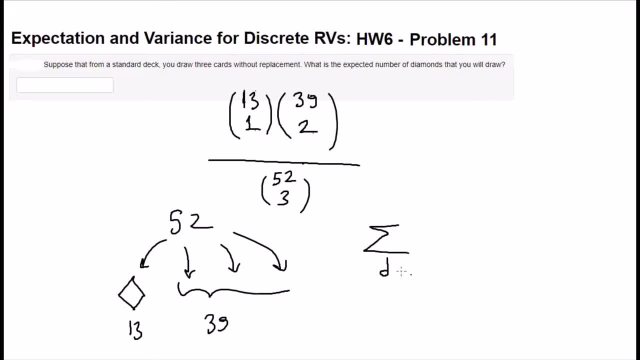 this as sum D from 0 to 3: D times 13: choose D times 39. choose 3. minus D: over 52: choose 3. so this is the answer and if you would like to expand this, let me expand this. so it's going to be the first card we are picking: 1 times 13. 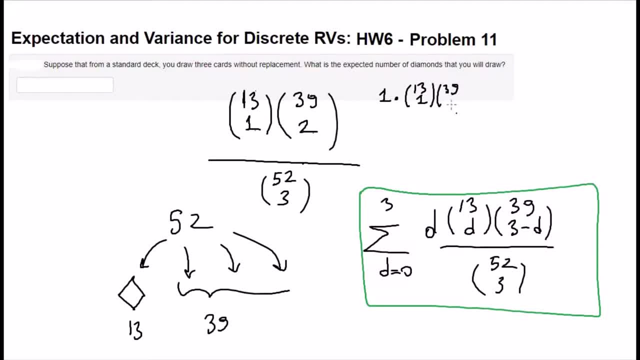 choose 1 times 39. choose 3 minus 1, which is 2 plus. second card is 2 times 13. choose 2 times 39. choose 1: 3 minus 2 is 1 plus. the third card is 13. choose 1. 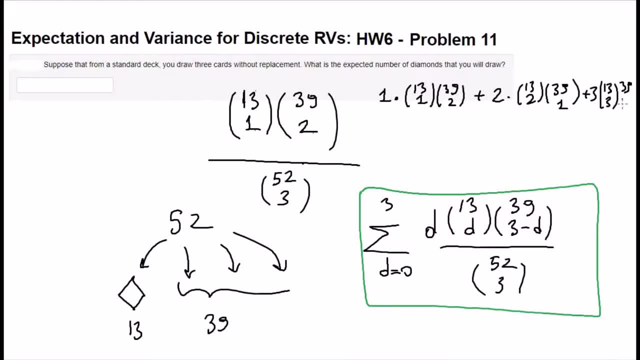 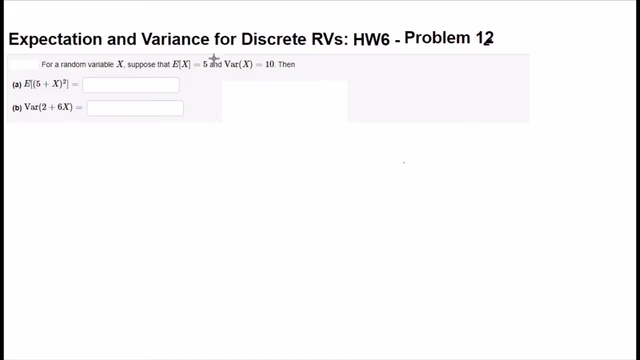 the 3 and 39, choose 0 and all over 52, choose 3. either this form or that form is the answer. problem number 12: for a random variable X, suppose that expectation of X is 5 and the variance of X is 10, then what is the expectation? 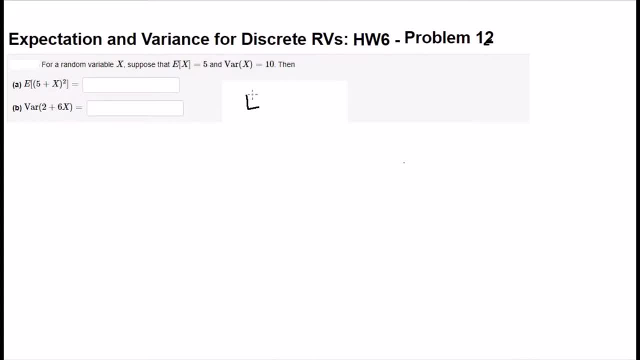 of 5 plus X, the quantity squared. so for this first, we are going to expand from 5 plus X, so we are going to do binomial expansion. so it's going to be 25 plus 10, X plus X squared, and that is equal to 25 plus 10 times expectation of X plus. 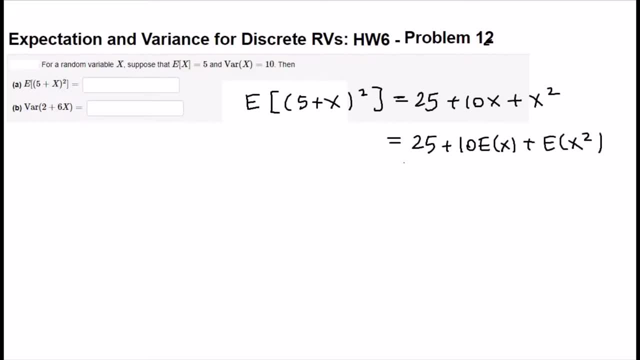 expectation of X squared. here we know expectation of X given 5, but we don't know expectation of X squared. variance of x, by definition, is equal to expectation of x squared minus expectation of x, the quantity squared. and from here, if we solve for expectation of x squared, 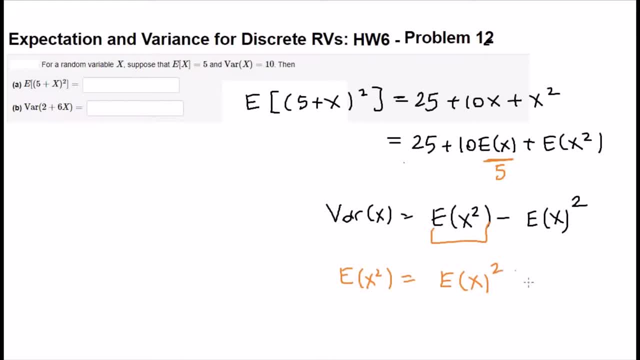 we obtain that expectation of x, the quantity squared plus variance of x. so we can substitute expectation of x squared as this: and when we switch variance of x to the right hand side, it is still positive, because variance is always positive by definition. now, instead of expectation of x squared here: 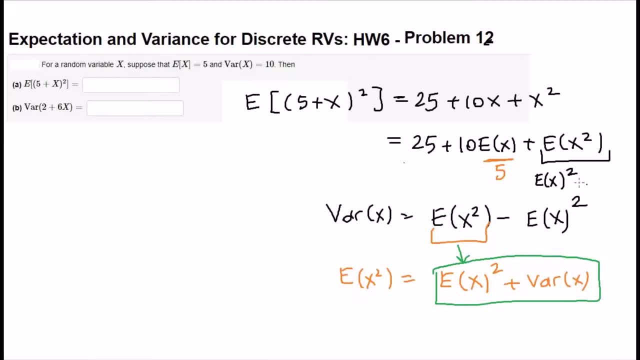 we are going to replace expectation of x the quantity squared plus variance of x, and we know the numbers. this is going to be 5 squared and this is going to be 10, and it's going to be 25 plus 10 times 5 plus 5 squared plus 10, we obtain 110. 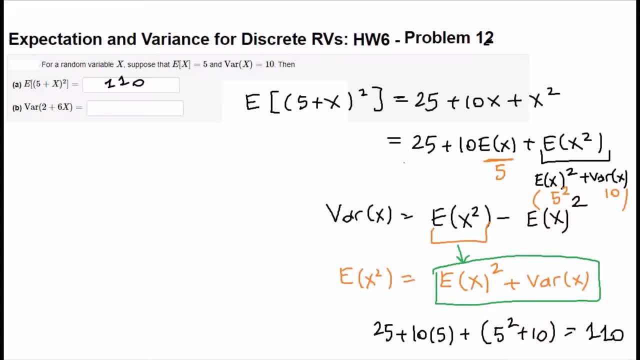 part b is asking variance of 2 plus 6 x. let's remember these two formulas: expectation of a plus b x is equal to the constant a plus b times expectation of x, and variance of a plus b x is equal to b squared times variance of x. so, knowing this, we can execute variance of two plus. 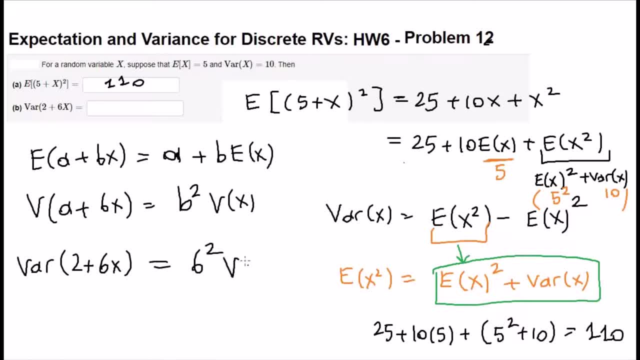 six x as six squared times. variance of x, which is six squared times. we know the variance of x, which is 10, so it's going to be 360.. problem number 11. let's change thening, sorry to the wrong function. problem number 11. 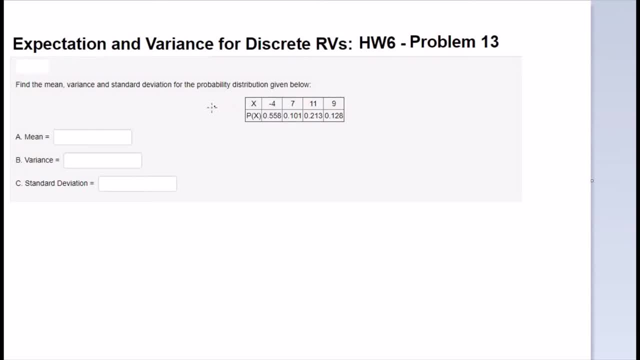 13. find the mean variance and standard deviation for the probability distribution given below. so mean or expectation by definition will be X times P, so it's going to be negative 4 times 0.558 plus 7 times 0.101 plus 11. 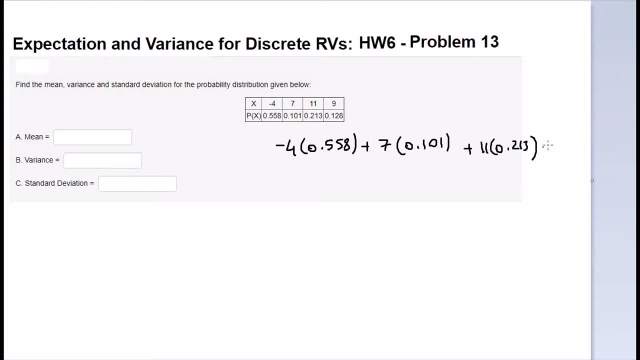 times 0.213 plus 9 times 0.128. so this is our mean or expectation. if you plug this in your calculator, you're going to obtain 1.97. variance, by definition, is expectation of x squared minus expectation of X, the quantity squared. so 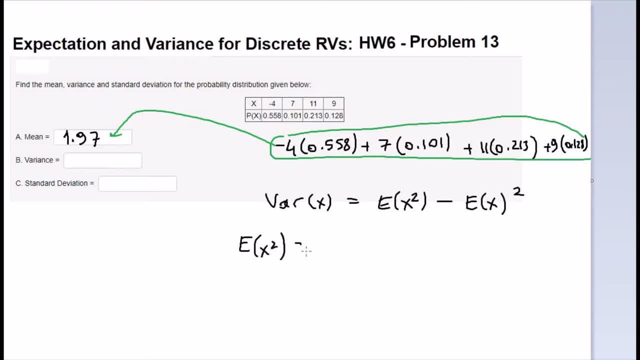 we need to compute the expectation of x squared. an expectation of x squared is exactly the same with the squared forms, and this value will give us 50 point 0, 18, and if this is 50 point 0, 18, and if this is 50.018 and if this is 1.97, then we square it and then what we're going to. 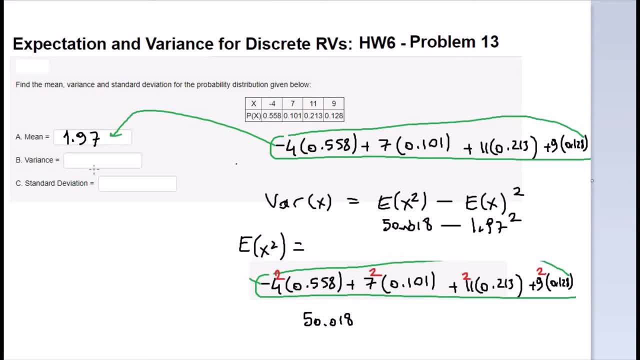 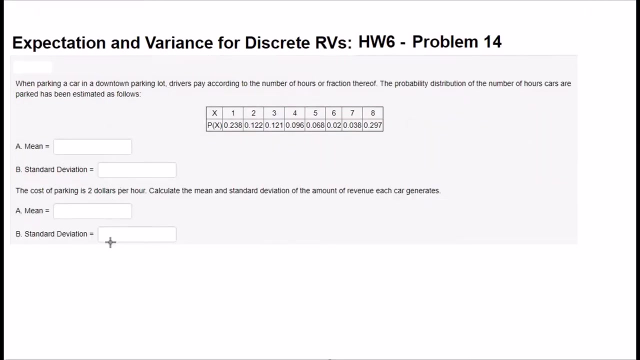 obtain is this value minus this value, which is 46.1371, and the standard deviation is the square root of the variance. so it's going to be 46.1371. so standard deviation Sigma is equal to square root of variance. problem number 14: when parking a car in a downtown parking lot, drivers pay. 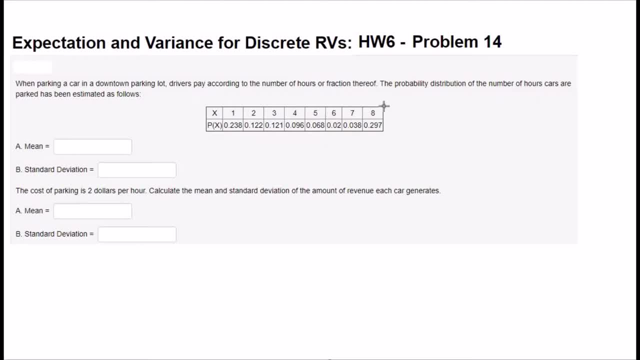 according to the number of hours or fraction thereof. the probability distribution of the numbers are given below. so we're going to calculate the mean standard deviation and the cost of parking- two dollars per hour- and the standard deviation of the amount of revenue each car generates. so let's 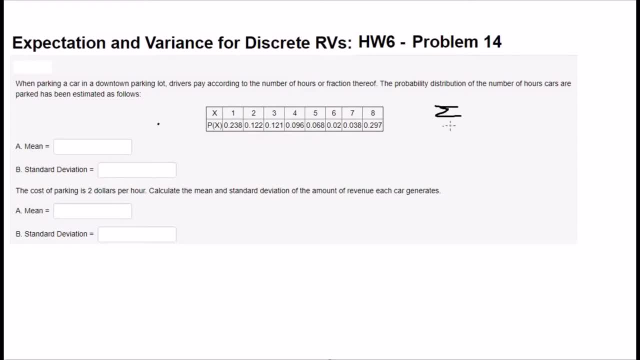 start with the definition of mean. the definition of mean will be X? I times P, I, which is X times P, here given explicitly. so it's going to be 1 times 0.238 plus 2 times the second probability, 3 times the probability of 3 plus 4 times 0.096. 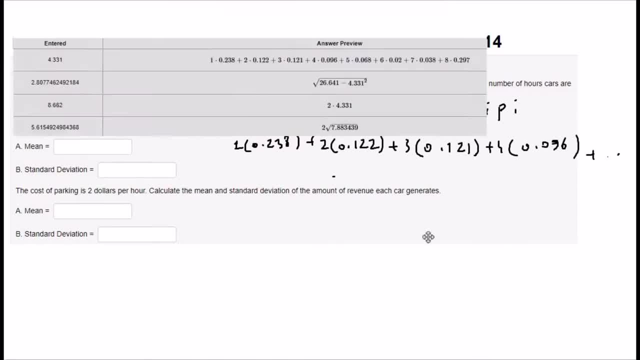 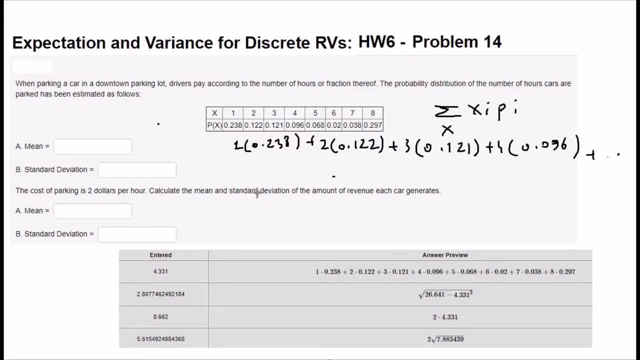 actually I did it, let me paste it. so it's going to be finally 8 times 0.297 and that number will give us the mean you and standard deviation is the square root of the variance. for variance, we need to find expectation of x squared and then subtract expectation of x. 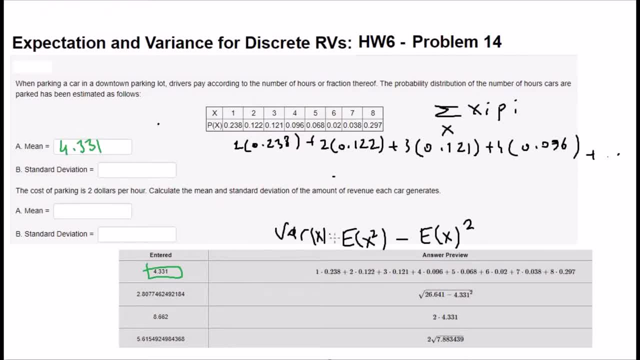 squared from expectation of x squared by definition. so expectation of x squared is- let me do it here: 1 squared times the probability. 2 squared 3 squared 4, 5. 1 squared times the probability that belongs to that x and that is this number, so 26.6. everyone is the expectation of x squared. we already. 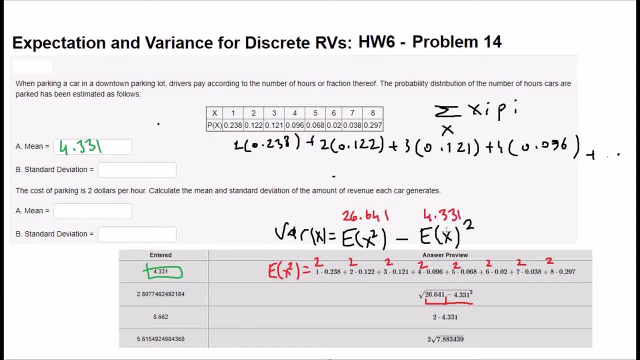 found the expectation, which is 4.3, 3: 1, and if we squared this two quantity we obtain the standard deviation. now the cost of parking, 2 dollars per hour, can be king is two dollars per hour. so if you multiply two times expectation dollar, two times the, 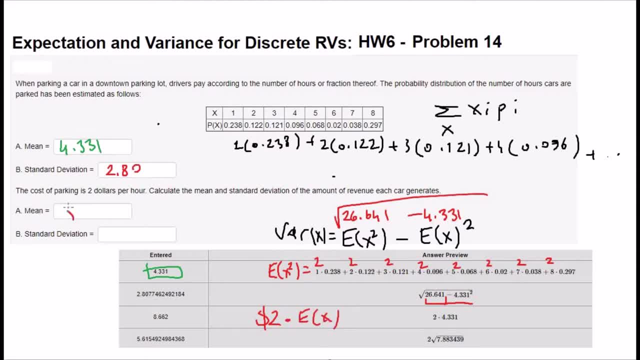 expectation will give us the answer, which is 8.662, and the standard deviation for this will be dollar, two times standard deviation, and standard deviation is this number minus that number. so it is this. so you can plug in either in this form or in that form. 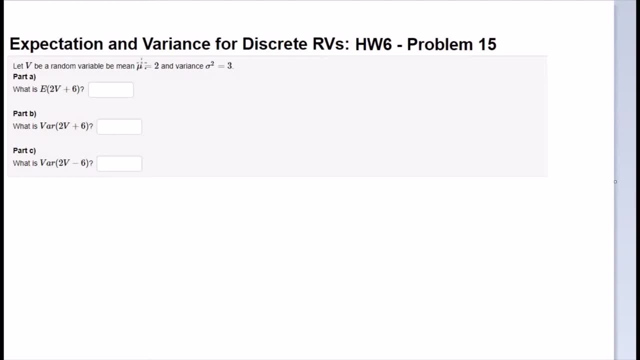 problem number 15, we were given expectation mu 2 and variance s3. so we're going to compute this, let's, let's remember the formula: expectation of a plus b x kind of argument- is equal to a plus b times expectation of x and variance of a plus b x is equal to just b squared times. 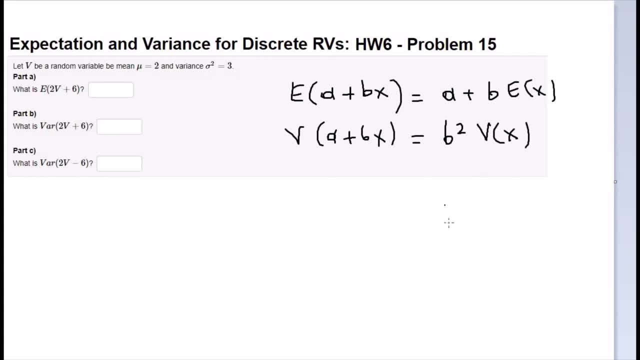 variance of x. so the constant here is ignored. so here expectation of 2v plus 6. v is here the variable, v not the variance. v is equal to two times v of x plus 6, so it's going to be two times mu. is given as two expectation plus 6. 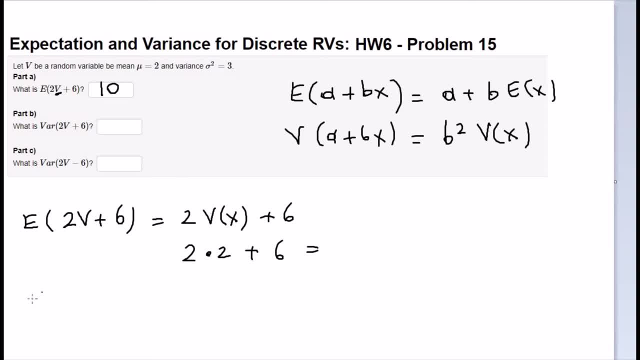 two times 2 plus 6, 10 for variance instead of 2v. you can consider it as to x, x, 2v plus 6 is equal to 2 squared times variance of v or x, whatever variable you consider. so it's going to be 4 times 3. 12 variance is given here and this is the same because that constant. 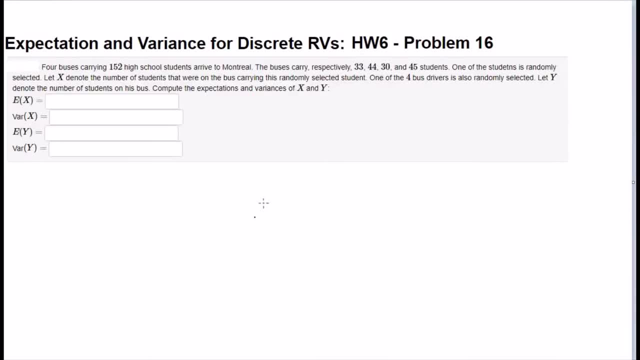 has nothing to do. problem number 16. four buses carrying 152 high school students arrived to Montreal. the buses carry respectively 33, 44, 30 and 45 students. one of the students is randomly selected. let X denote the number of students that were on the bus carrying this randomly selected. 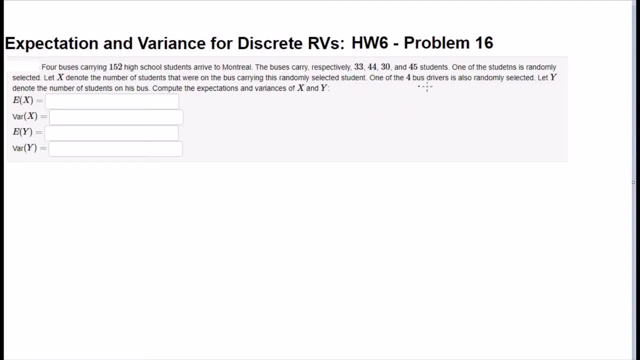 student selected student. one of the four bus drivers is also randomly selected. let y denote the number of students on his bus. compute the expectations and variance of x and y. so for random variable x, we have 30, 33, 44 and 45 students, total 152 students and the probability: 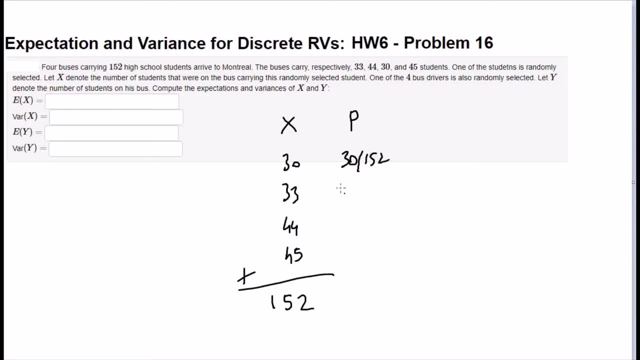 for this is 30 out of 152 and probability for this is similarly this and expectation will be x times p plus x times p, plus x times p, plus x times p. so the expectation here will be 30 times 30 out of 152 plus 33.